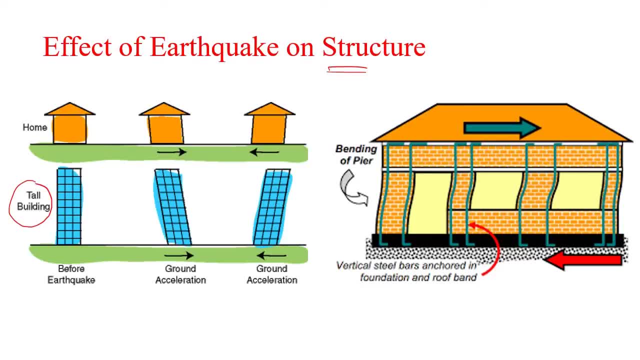 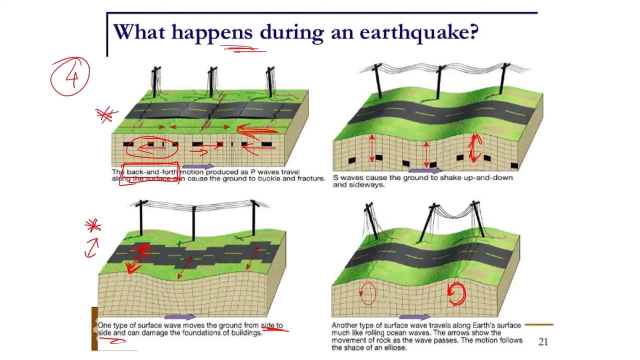 this particular tall building. this is the case before earthquake. the ground is in rest and, as a result, you can see that the whole structure is aligned vertically compared to the ground. but once the ground start to accelerate- here you can see that ground accelerate horizontally during the earthquake. so what will happen? the ground start to accelerate. 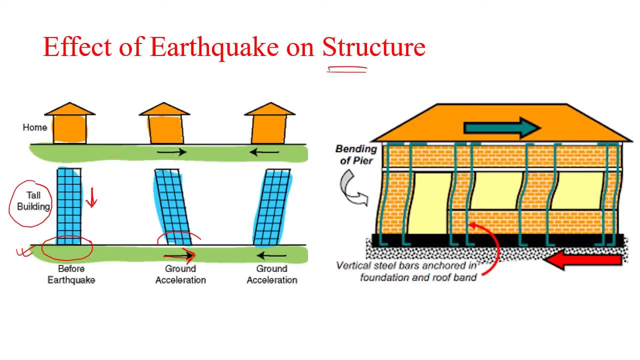 horizontally and the lower part of the building simultaneously accelerate along with the ground, because this is attached with the ground, but the top part of this building is far away from this ground. as a result, there is a drift. okay, this is. this difference of lateral movement is known as lateral drift, and you know that if you consider any 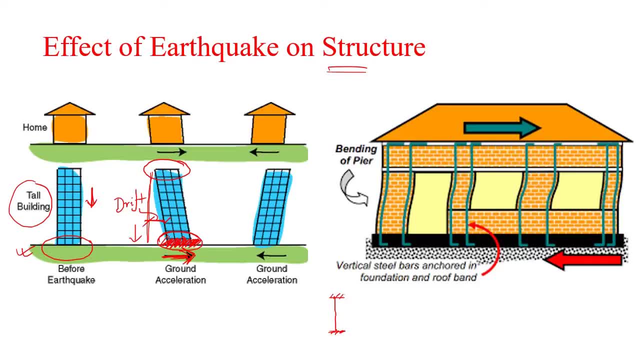 column or beam. that is fixed, okay, but the one end is deflected. what will happen? there is a moment caused due to this deflection, right? i think you know the value of this moment, that is 6 e. i delta by l square, something like that, right? so due to this drift caused by this ground acceleration, 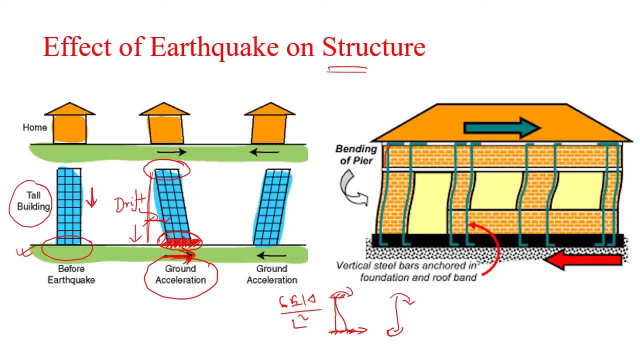 the vertical member as well as the horizontal member of the building, as here you can see, is subjected to extra stress due to this differential drift. okay, or you can say, this vertical member or this particular column is subjected to extra moment caused due to this ground acceleration. okay, so we are interested about earthquake load because it caused the drift. 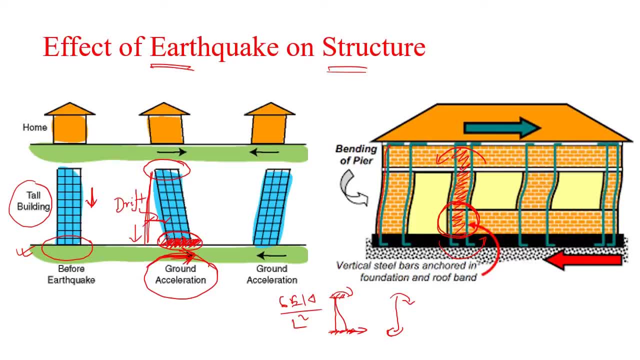 within the structure due to its ground acceleration, okay, and due to this differential movement from top to bottom, there is a extra stress within the member right. so this is the main effect of earthquake on any structure. so here you can see, due to this ground acceleration, nothing but a. 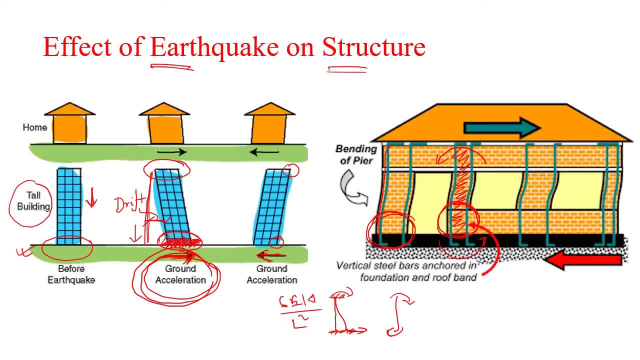 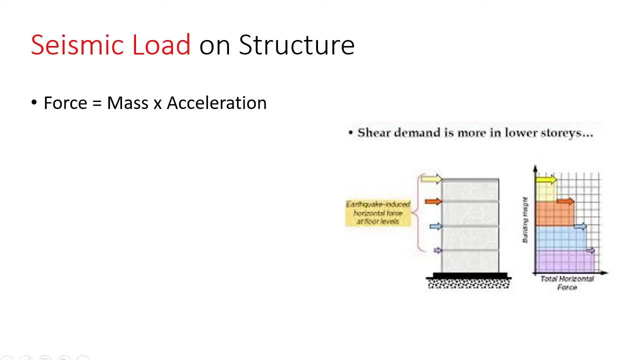 lateral load is being generated. okay, so ground is moving from this side to this side, but above the ground, we can say that a lateral load is being applied from this side to this side right now. what is the magnitude of this lateral load? simply, the load or the force is nothing but the mass time. 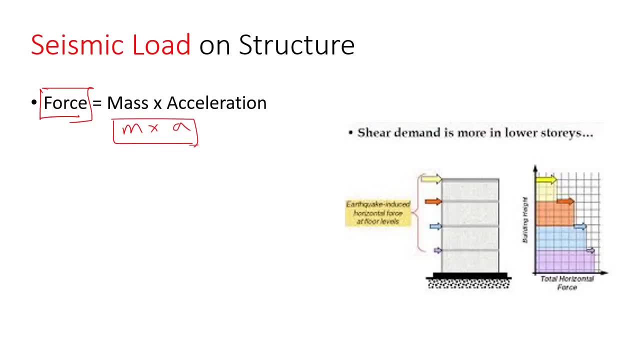 newton's law, right, simply from newton's law, the force that is being applied is equals with mass on which the force is being applied, times the acceleration. okay, so now you can see that as the ground moves, okay, the acceleration is same for every point, right? but the mass? if we consider the 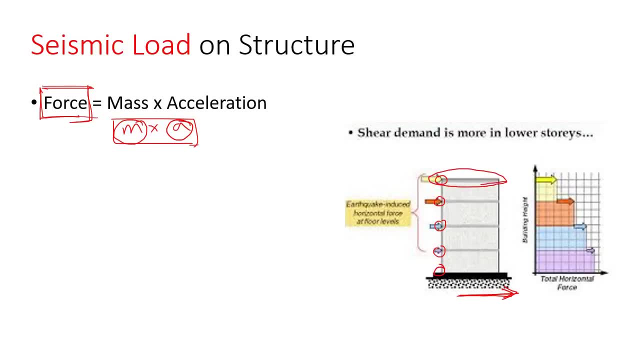 mass of this particular point. this is nothing but the weight of this zone. but the mass of this point is simply the weight of all the floors above it. as a result, you can see that at the roof level the lateral load due to the seismic is least, but at the base level or at 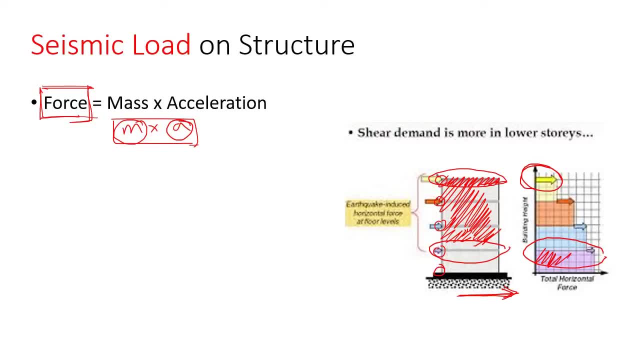 the first floor or the ground level. it is maximum because at this point the mass is narrowed when it comes down. that is the interaction, right? the rise of the partial� colors, that is veryangs, let's say that Public. so now there should be no gap between the of the block of. that is not. it has area level, all right. 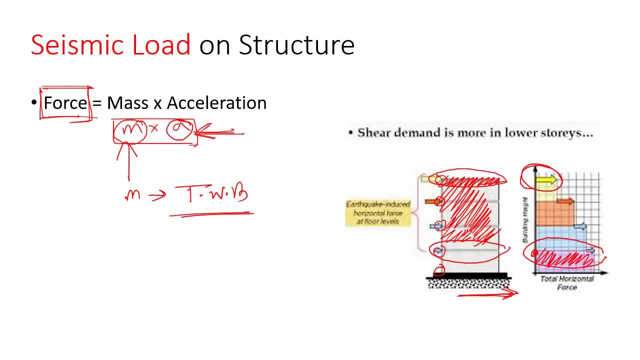 so in how to calculate the crianças equation. so the problem is that the question is how to calculate the analysis of the uncertainty of the owns' fairly under the gravity of the precal Alaska and dick's- but he's been very close to too speed- and how to calculate the sum of the total weight of the whole building. 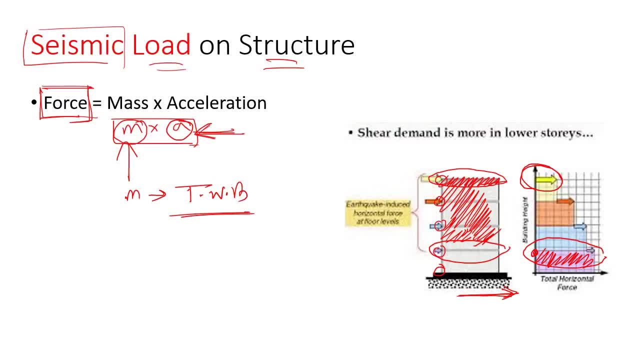 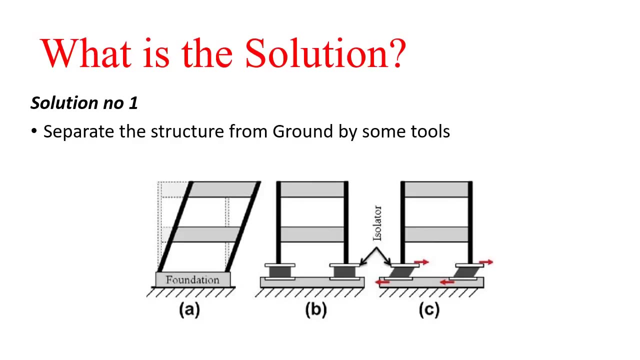 load, or why the load varies right now. what is the solution? simply here you can see that every problem is being created from this ground, right? so ground is the source of all problem. so the very first solution is simply separate the structure from the ground. now you can ask me: how is it? 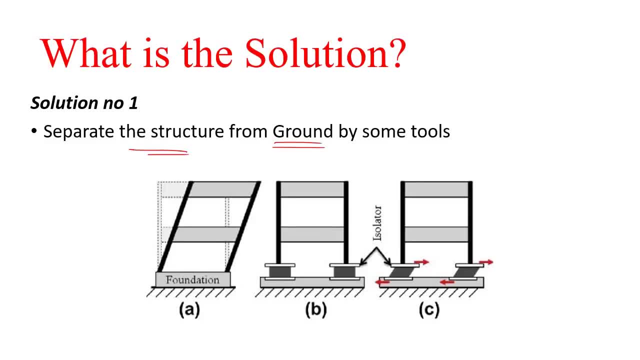 possible. normally, we build each and every structure over the ground. well, that's very correct. but if we install any particular tools, like this elastomeric bearing, what will happen once the ground start to move? okay, this elastomeric bearing will deflect, like this, and the structure will remain in its own shape and there will be 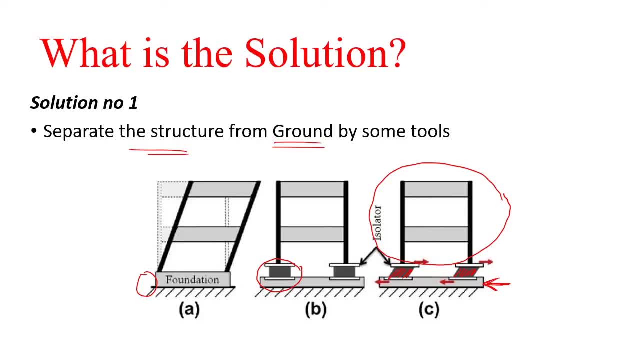 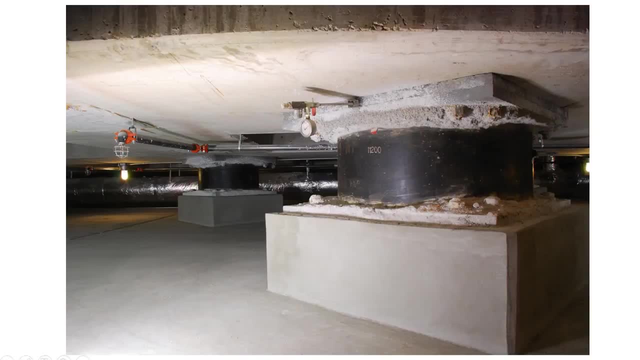 no problem with that. so now let's see how to build a structure from this ground, such lateral force. now, if you have any confusion about how, under the lateral load, elastomeric behave like this, i have already made video on this elastomeric bearing topic. okay, you can go to the playlist. you can watch it also. right, so in real life, this is the building. 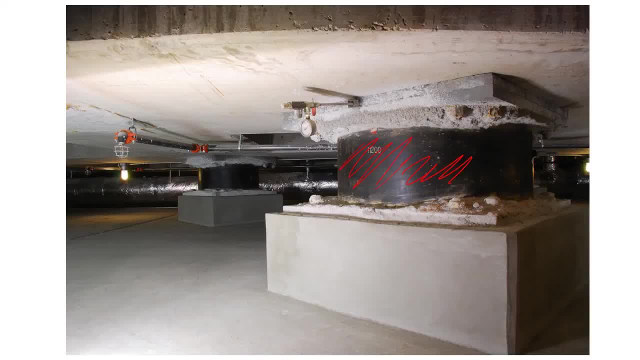 basement, and here you can see, we have installed this huge elastomeric bearing. okay, so once the ground start to accelerate during earthquake, what will happen is that the structure will happen. simply, this elastomeric bearing will deflect. first, like this, okay, and the top of this. 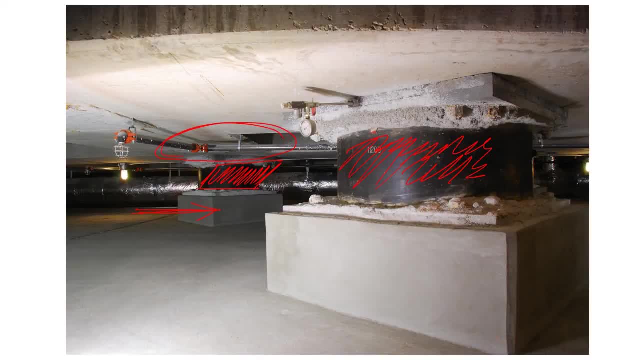 structure will be unaffected. okay, so this is a great idea, but this is also a very much complex as well as not that much economical for a smaller structure. okay, let's say you have a simple steel pipe rack, so of course there, you are not going to install this type of 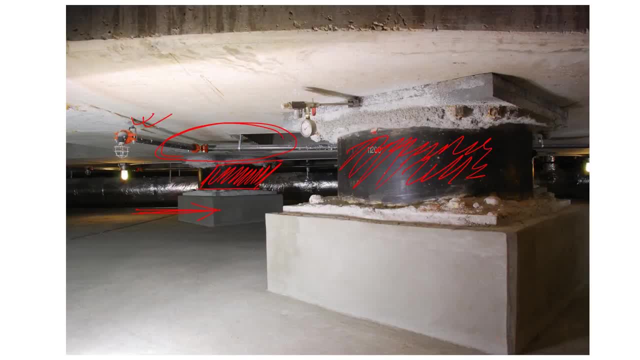 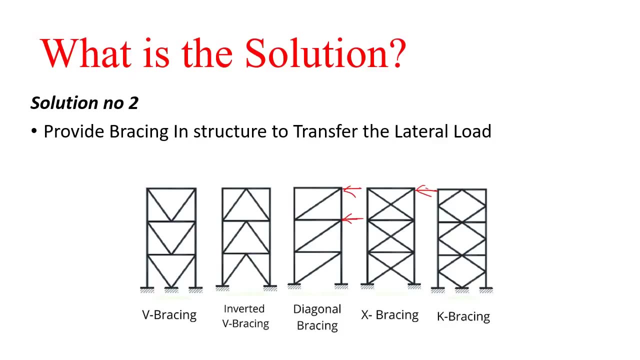 expensive steel pipe rack. you are not going to install this type of expensive steel pipe rack wearing at the basement. so in that case, what is the solution? simply, if you have lateral load like this, like this, due to this seismic load, what you have to do? you have to transfer. 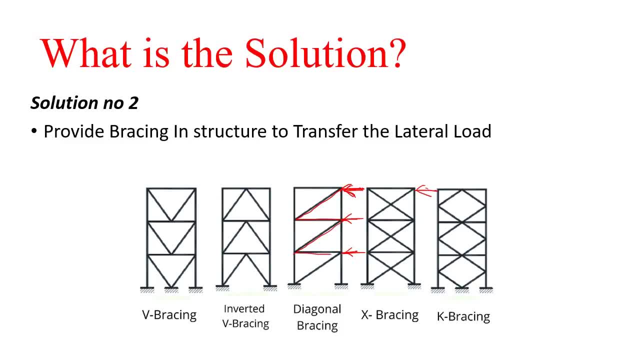 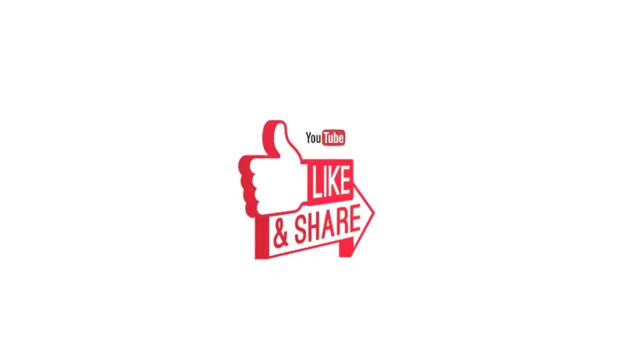 this lateral load, through this racing right to the foundation and your purpose is solved. so that's it. if you like this video, don't forget to share it.